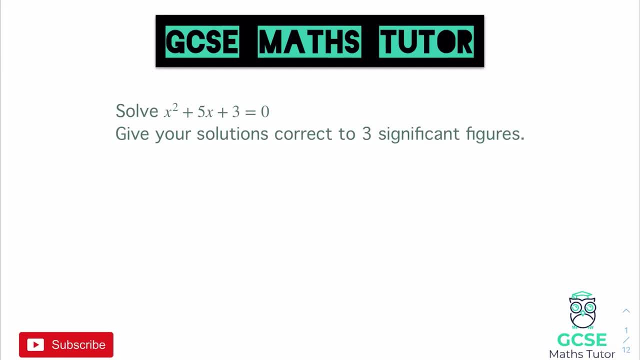 created. I'm going to briefly talk about where it comes from, but if you want to have a look at how it's created, I'll link that video in the description for you. and it's a nice quick little video if you just want to see how we actually get or form that quadratic formula. Now for any quadratic we're. 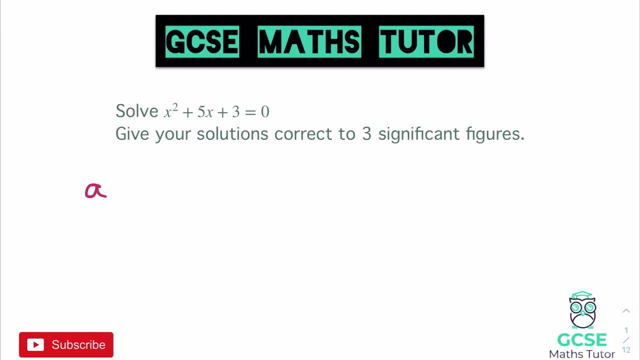 looking at the quadratic, when it is in this form, ax squared plus bx plus c equals zero. So we're having a look at these numbers here that are in front of the x squared, which in this case is what we call a, in front of the x which we call b, and the number at the end, which we call c. Now what? 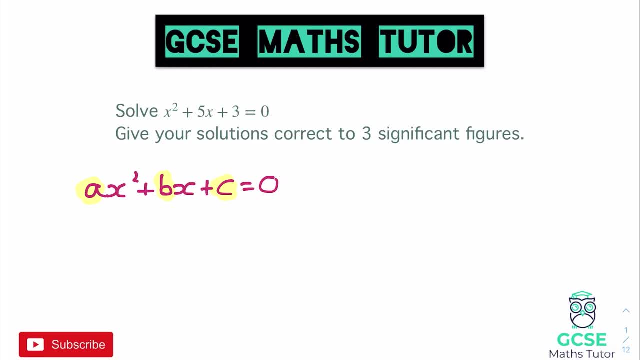 happens is when this piece here is rearranged, it forms the quadratic formula and, as I said, if you want to see how it turns into the quadratic formula, you can go to the link in the description for the quadratic formula. I'll link that video at the top of the description so you can have a look. 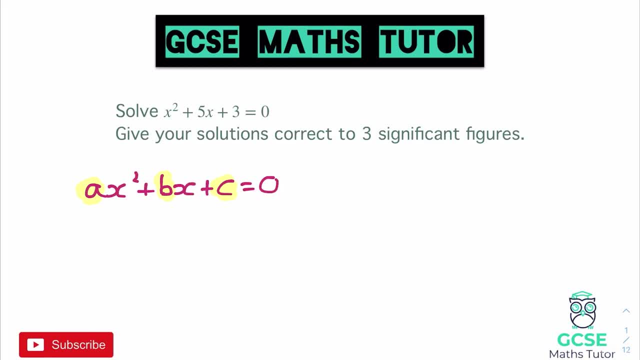 But when we rearrange this- okay- and there's quite a lot of steps in order to do that- we get this formula okay, and it's x equals okay, and on the top of this fraction that we're going to have here, we get minus b plus and minus the square root of b, squared minus 4ac, all over 2a. 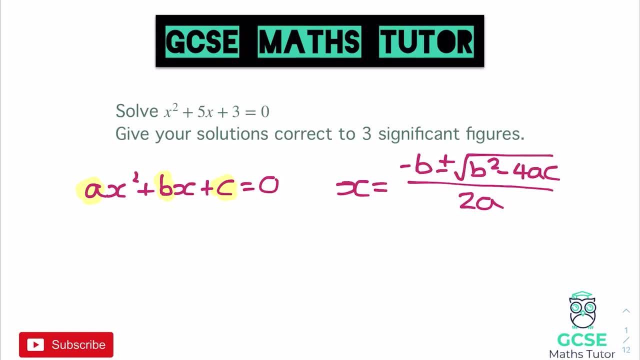 Now that there is the quadratic formula and it allows us to do a lot of things To solve a quadratic without actually having to factorise it- okay, because the times that we would use this is when quadratics cannot factorise. Okay, we could use it for quadratics to factorise, but it's a bit of a longer process if you are able to factorise it. 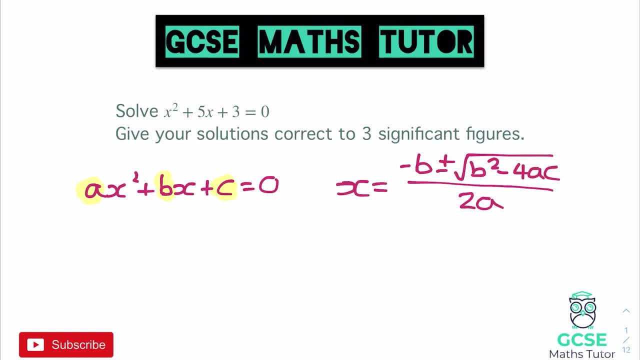 So, again, if you want to see how this is actually created, I'll link that in the description. but for the purpose of this video we're going to be using this formula, so make sure you have that one written down over there. x equals minus, b plus and minus the square root of b squared minus 4ac all over 2a. 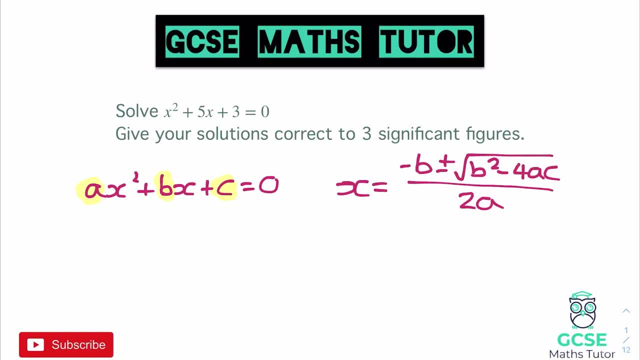 And for the purposes of the GCSE exam, you do actually have to remember this formula, so it's worth writing it down and writing it down a few times until you're able to remember it, Although the best way to remember this is just to practice some questions. So for this one here, all we need to do is we need. 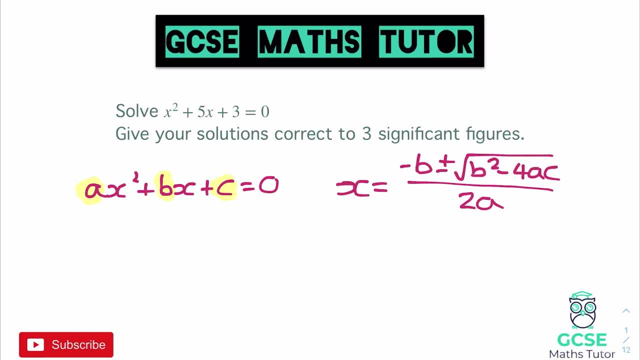 to identify what the values of a, b and c are, because you can see in the formula we've got a's, b's and c's. Now that's easy enough. all we have to do is have a look at our quadratic. but one thing that's really. 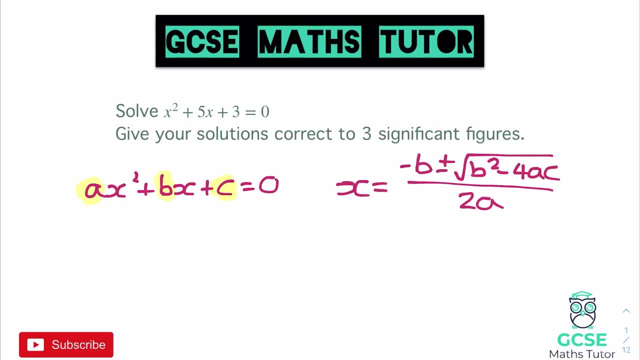 worth noting here is that the quadratic has to equal zero. That's absolutely key for a quadratic, because what actually a quadratic relates to is the number of times that we have to factorise it. It's a quadratic graph, and if I was just to draw a basic little sketch of a quadratic graph, it would: 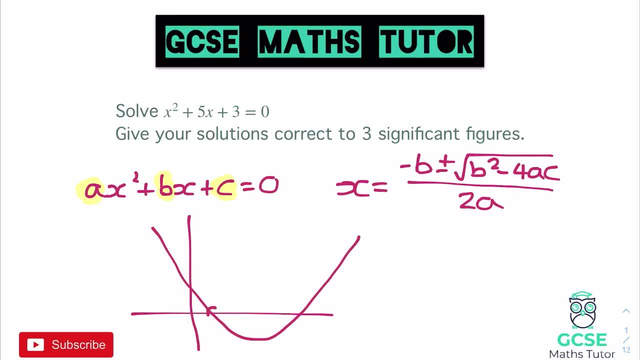 look something like this and what we are finding is these two points here where it crosses over the x-axis. Okay, and in terms of a little logical reason here, when it equals zero is when y equals zero, and when y equals zero, that's anywhere along the x-axis and I'd almost refer to it as being 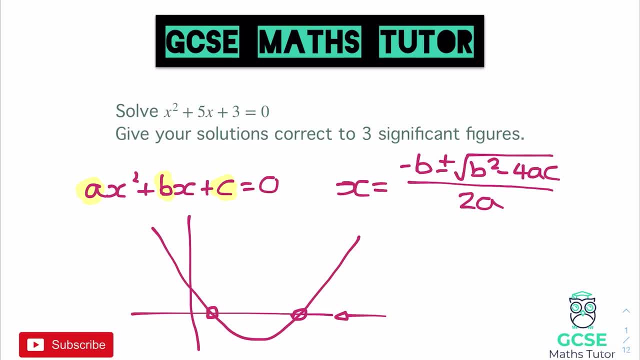 ground level. Now, if it wasn't equal to zero, let's imagine it was equal to five or something else. If it was equal to five, it would be equal to zero. So if it was equal to zero, it would be equal to five. What we'd actually be finding is the points here where it crosses through, when y is five and 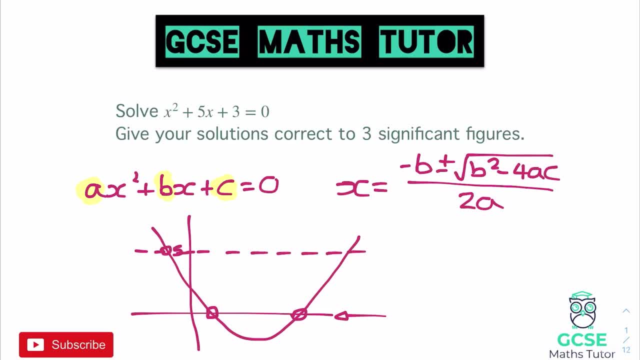 that would obviously give us two very different solutions. It would give us this one here and it would give us this one here, and we're looking at where it crosses the x-axis for those solutions, or sometimes called roots, as well when we refer to the graph. So that's very key. they all have to. 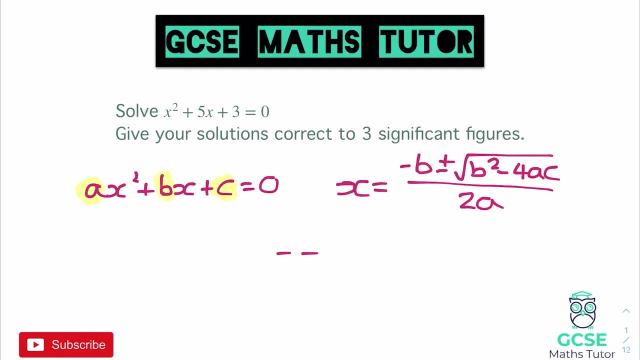 equal zero. For the purpose of this video, they are already going to equal zero, but just thinking about the future of this topic, the quadratic has to equal zero in order for us to solve it. So let's have a look at actually solving this question then, and we'll pick out our values of a, b and c. 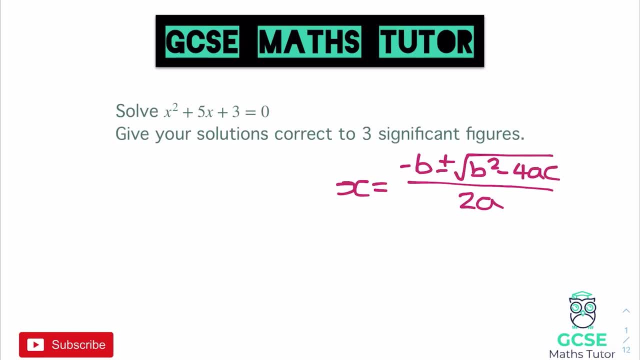 and let's have a look. So for this quadratic that we have here, x squared plus five, x plus three equals zero. The number in front of x squared obviously isn't written and that means that a is equal to one. it's a one x squared. The number in front of x there is positive five. so I'll just 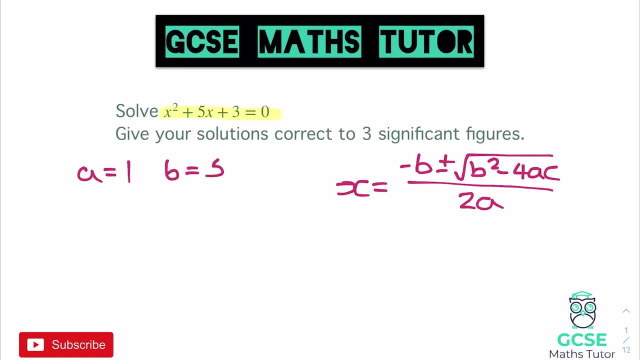 write: b equals five and the number at the end is the three. so c equals three. Now, from there, all I have to do is put, put it into the quadratic formula. So if we're getting about the x equals for second, let's just put all the numbers in place of the formula and see what we get. So b is five, so 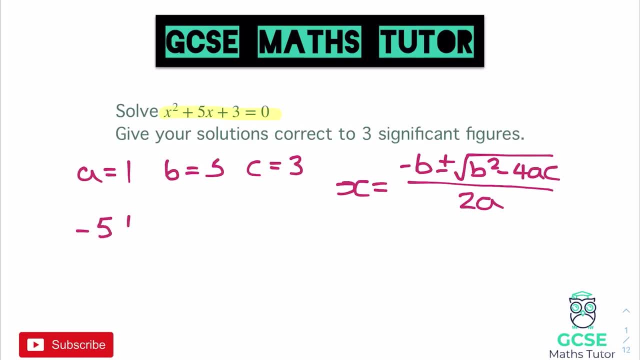 we have minus five on the top, as it's minus b plus and minus the square root of five squared minus four ac. Now whenever I'm squaring something in my calculator, I always put it in a bracket. so let's put five in the brackets squared. I'll talk about that later on a later question. 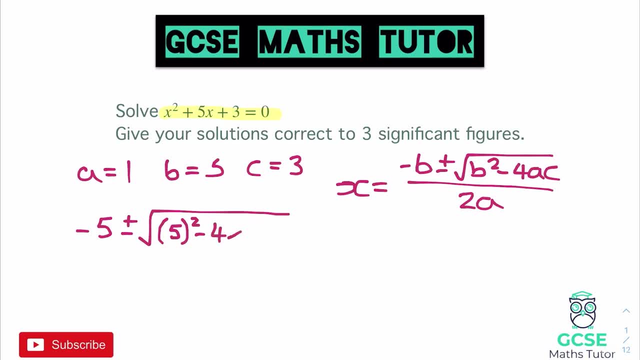 Take away, and then we have four times one times three, And that's all over two a, which is two ones. so two I'm going to put two times one, though just to emphasise the fact that I've substituted that one in place. Now, there we go, we've put it into. 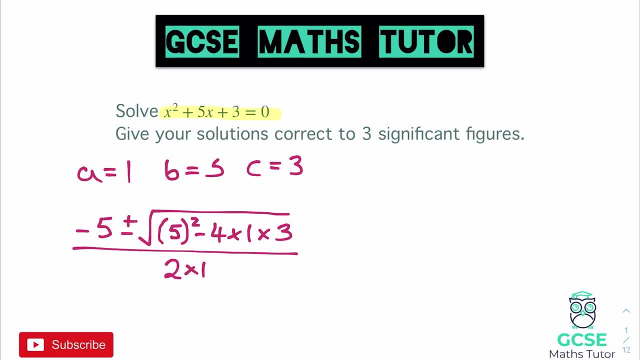 the formula. Let's get rid of this formula now, and we just need to actually get our solutions. Now. one thing you'll notice is obviously we have this plus and minus, and that's because the square root of a number always has two solutions. Just thinking about the square root of 25, for example. 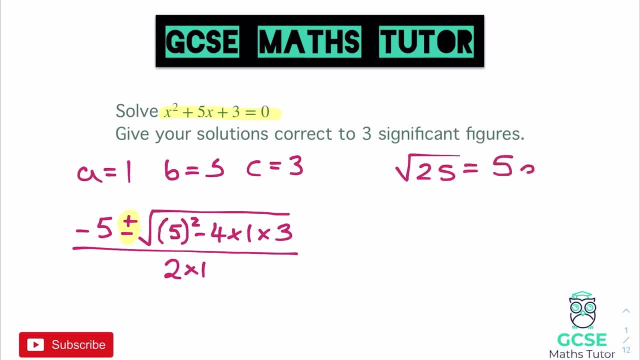 the answer, which most people will say, is five, but it can be done in any other way. So I'm going to go back into my calculator and change it for a minus. Okay, so typing this into a calculator then. So I'm going to take 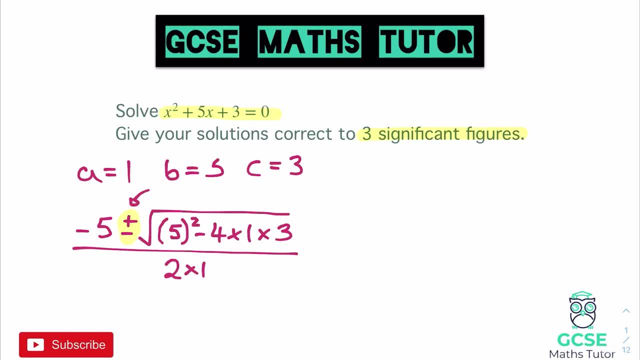 the minus five and I'm going to use the negative button, obviously, rather than take away, to emphasise it's a negative. So negative five plus. and then I'm going to do the square root in brackets: five close, bracket squared. take away four times, one times three. 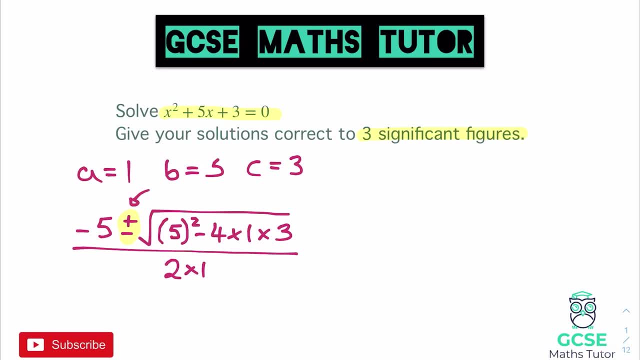 and on the bottom of the fraction, two times one, which is two. So I'll just put two press equals and we get an answer. Now just to emphasise that that's the positive one. just by my working out here, I'm just going to put a plus sign. so I know that's the one I've done. 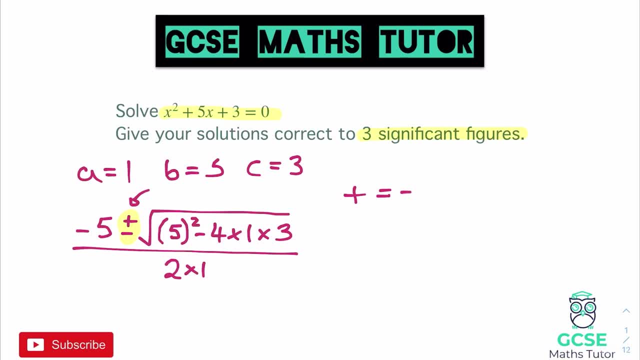 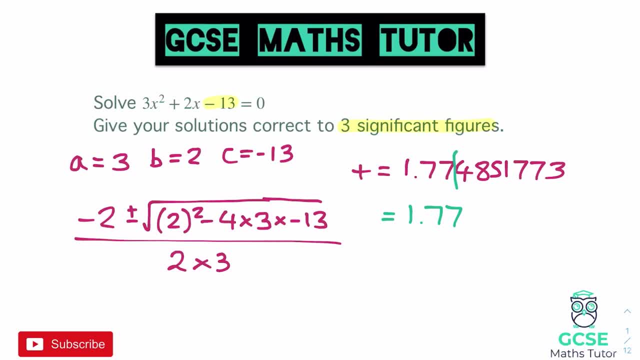 us put a takeaway in there and press equals again. and here we go. we've got our second value here. so for our negative value we're going to get 2.44. so I haven't put the negative sign in there, it's negative 2.44. so we get negative 2.44151 and then 844. there we go, and again three significant. 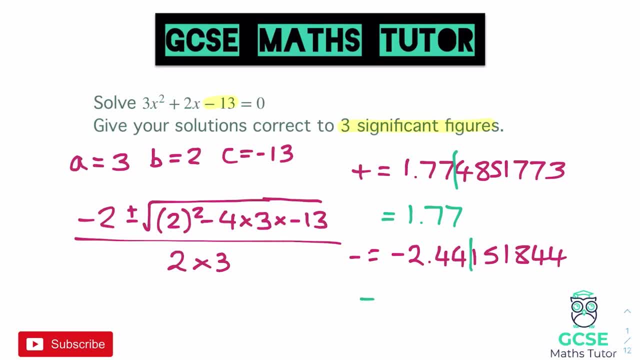 figures, so 244, and again the one that is not enough to round it up there. so our final answer is negative 2.44. and there we go. there's our two final answers: 1.77 and negative 2.44. now again, you're going to have a go. now. one thing you are going to need is, obviously, your calculator. 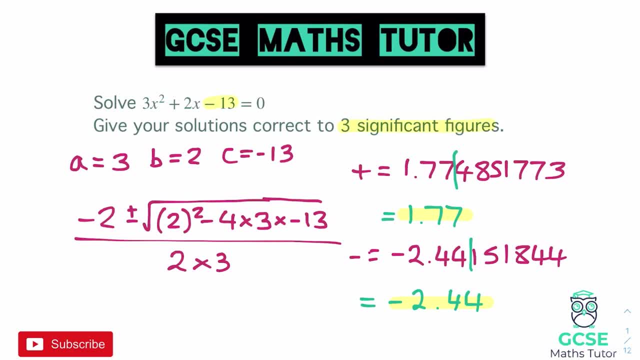 which I hope you've already been using, and obviously I would suggest that if you don't already, it'd be definitely worth getting yourself a Casio calculator. I've linked a few calculators in the description below. if you want to check some of those out, it's definitely worth. 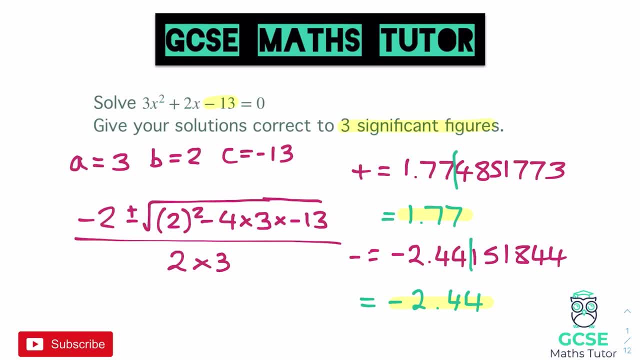 having a look at them, and I'll see you in the next video one. you get this sort of dual level ability to be able to do this. if you don't have one of those calculators, though, you're going to have to type the entire top line into a bracket, potentially. 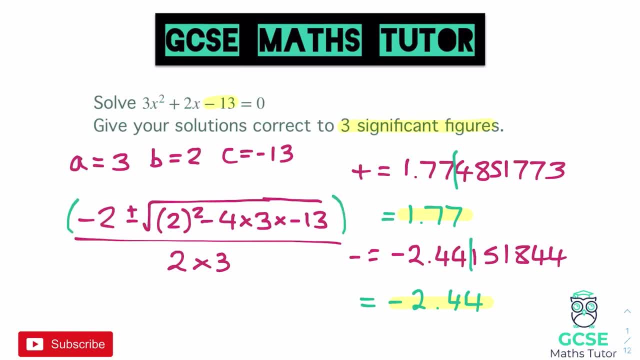 if you're using a single line calculator and then pressing divide by and then whatever's on the bottom. that is only going to be necessary, though, if you only have a single line calculator. obviously, if you're thinking about doing your GCSE exam relatively soon, it's definitely worth. 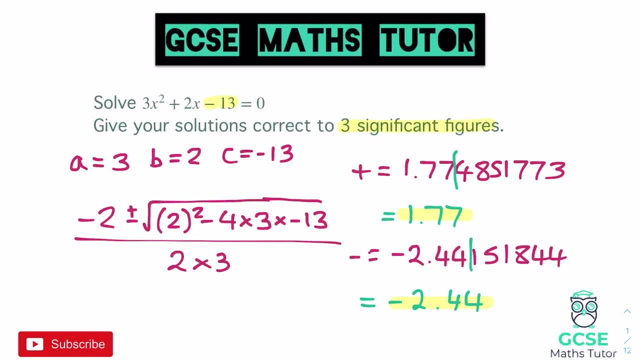 getting one of these Casios, particularly for the higher paper. I think it's pretty much essential. it just gives you that little bit of an advantage when you're doing things like that, like this. but there we go. that's in the description, so you can check that out if you don't already. 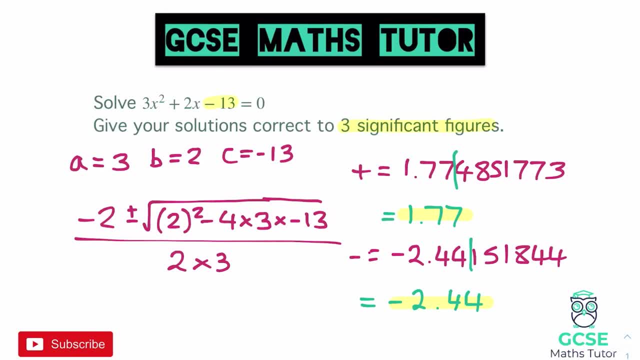 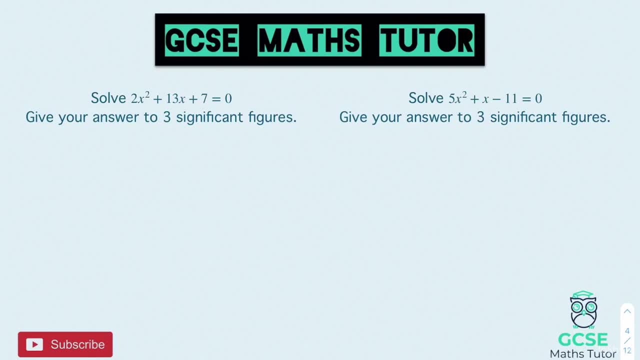 have a Casio calculator, and here we go. we're going to have a go at a couple of questions, okay, so here's your two questions, so pause the video there, have a go at getting the answers for both of these and we'll go over the answers in a sec. okay, so for the first one then. so we have. 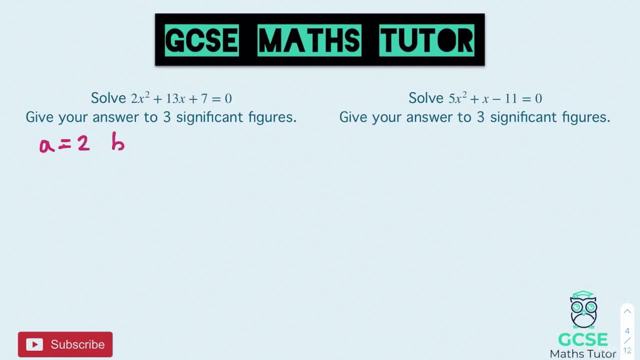 a equals 2, we have b equals 13 and we have c equals 7 and putting that into the formula, we get minus 13, plus and minus the square root of 13, squared minus 4 times 2 times 7, and that's all over 2a, that's all over 4, and let's type this in: 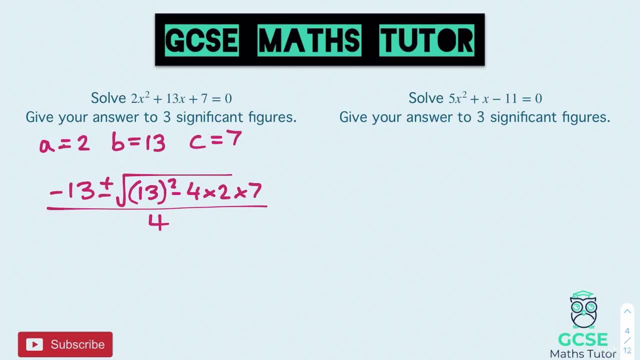 so negative 13 plus the square root of 13 squared, take away 4 times 2 times 7 and that's all over 4 press equals, and we get our first answer here, which is- and this is for our positive value- negative 0 point 5, 9, 2, 4, 6, 3, 5, 4, 6, 8. always long decimals there, and for our negative one, we'll round that. 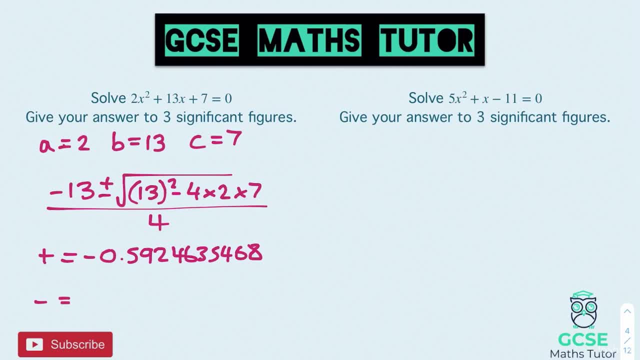 in a sec, our negative one there. change that plus for a minus. there we go and we get our second answer, which is negative: 5 point, 9, 0, 7, 5, 3, 6, 4, 5, 3 and again let's round these. so for the first one we'll chop that after the 2, so that becomes negative. 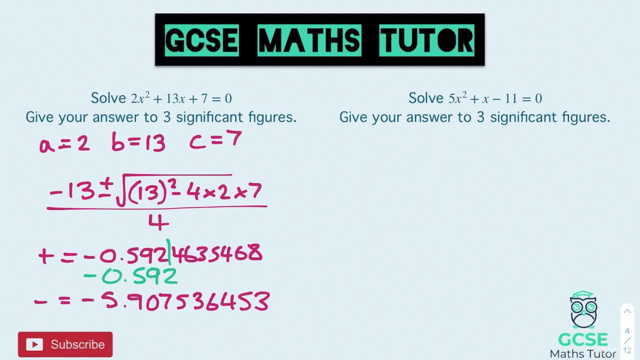 0 point 5, 9, 2. and for the last one there, chop it: after the 0, the 7 is going to round that up. so minus 5 point 9, 1, and there we go. we have our two answers, there we go, so there's our first one. 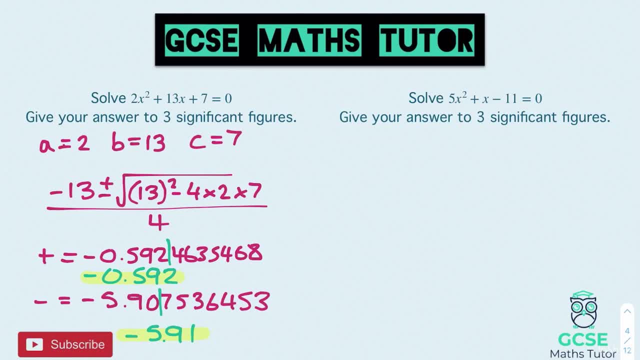 let's have a look at our next one here, where we have a negative c value, so a is, this time is 5, b. we don't have a number in front of x, so b equals 1 and c equals negative 11, and again let's plug that into our formula. so we have minus b. 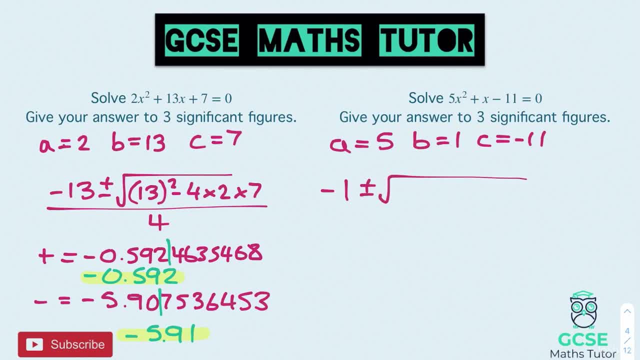 so minus 1 plus and minus the square root of 1, squared minus 4 times a, which is 5 times c, which is the negative 11, and let's put that all over 2a, which is 2 times 5, 10, and let's plug that into. 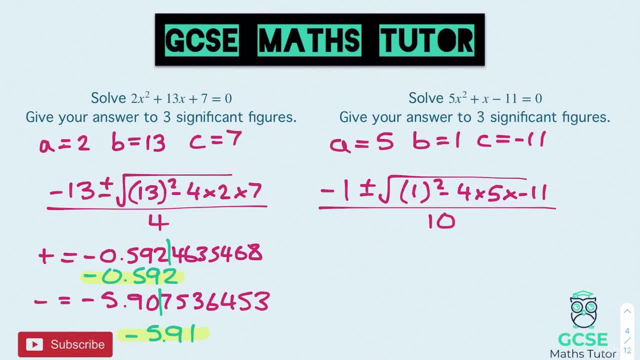 our formula so negative: 1 plus the square root, and again I'm going to put 1 squared in brackets, even though 1 squared is 1, take away 4 times, 5 times minus 11 and that's all over 10 pressing equals and we get our first. 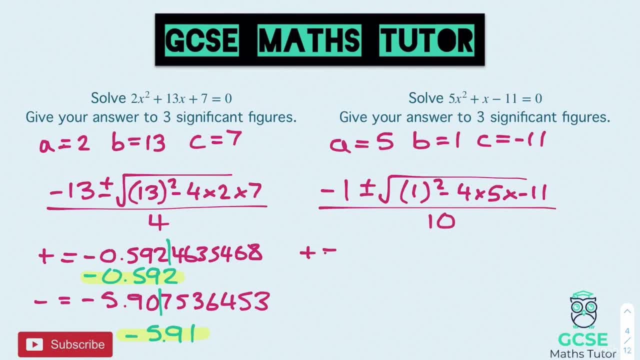 answer for our positive version or our plus version there, where we're using the plus sign 1 point 3, 8, 6, 6, 0, 6, 8, 7, 5 and let's do our negative one. so for our negative here, let's type: 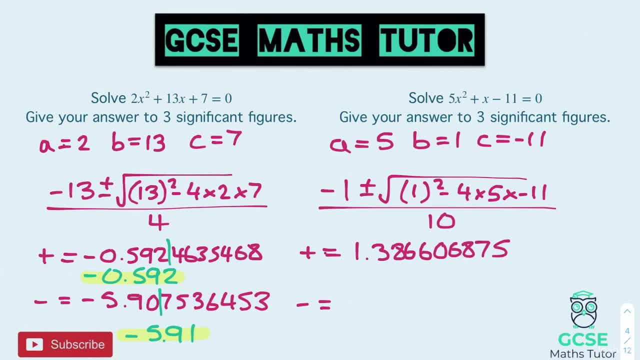 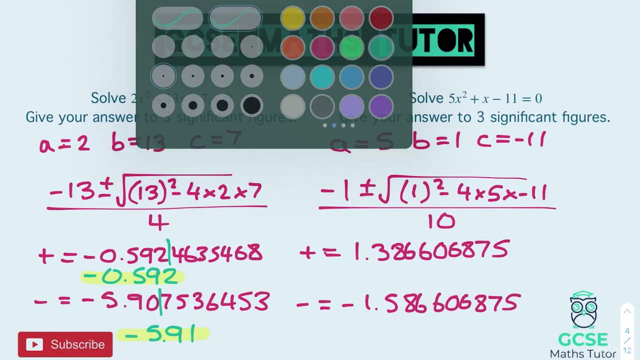 let's go back in and change that plus for a minus and we get a value here of negative 1.58. 6, 6, 0, 6, 8, 7, 5. okay, and let's round both of these. so 1, 3, 8. the 6 is going to round that up, so that's going to be. 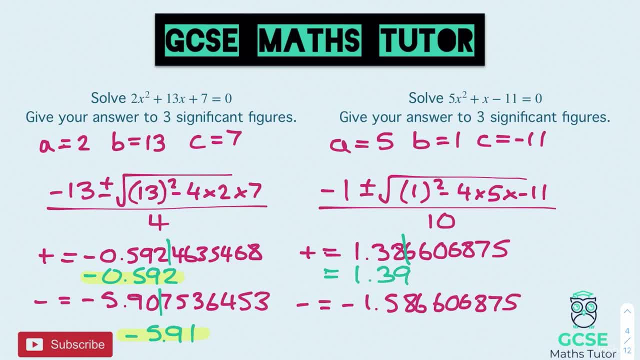 1.39, and for the second one here, 1, 5, 8, and again that 6 is going to round that up, so that's going to be negative 1.59. and there we go. there's our two solutions and there's our two questions. 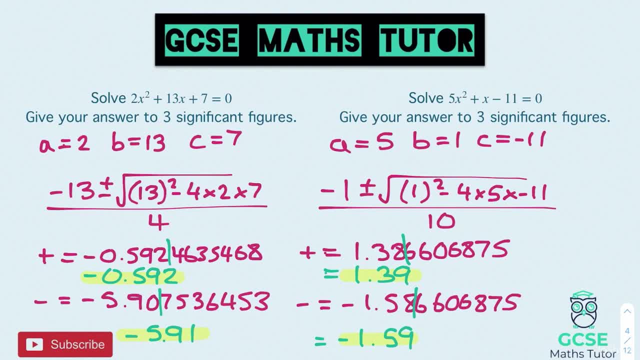 completed now, obviously, both of those there. we have not yet had a negative b value, so we're going to have a look at- now is one question with a negative b value, and then we're going to have some non-calculator versions, so let's have a look at those now. okay, so in this one here, hopefully, 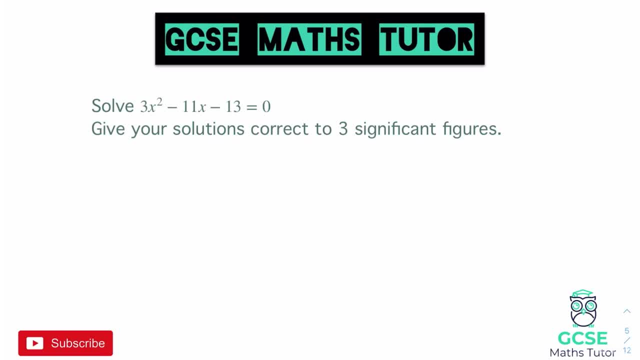 you can already see from the first line that we're going to have a negative b value. we're not really going to do anything much different here. we just need to be careful with that b value. we're going to have a look at how it changes slightly. 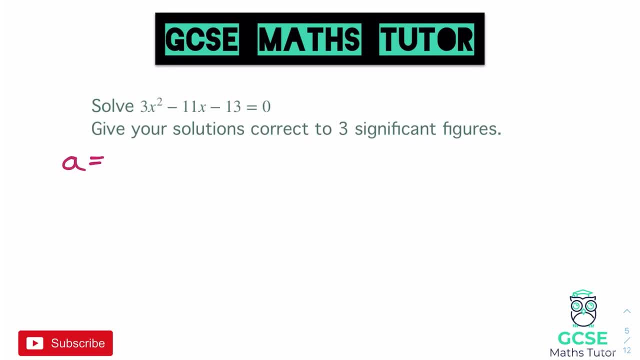 here. so for our value of a we get 3. for our value of b, this time we have negative 11 and again we've got a negative c. value c equals negative 13 and when we put this value in, as we have negative b on the start of our quadratic formula, that's going to change our negative 11 to positive 11. 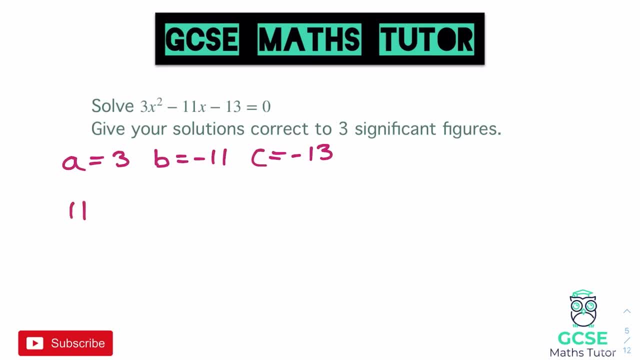 so, on the top, we're going to have positive 11 this time, as that double negative there is making it into a positive 11. so we're going to have a negative 11 this time, as that double negative there is making it into a negative 11 this time, as that double negative there is making it into a negative 11. so we then still have the plus and minus. 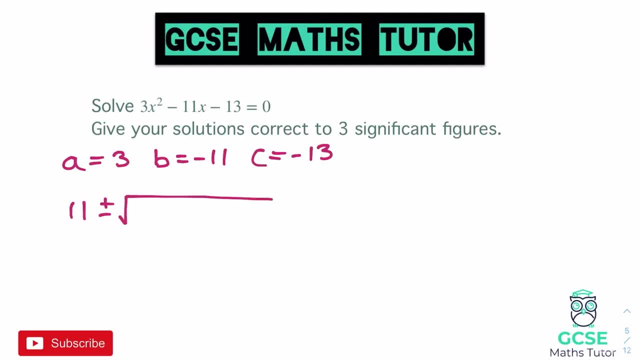 and then we're still going to put our b value into a bracket. now this is really important, where this really makes a difference, because if you don't put this negative 11 into a bracket, what your, what your calculator will do is it will do a negative 11 squared, but not properly do a negative 11 squared. 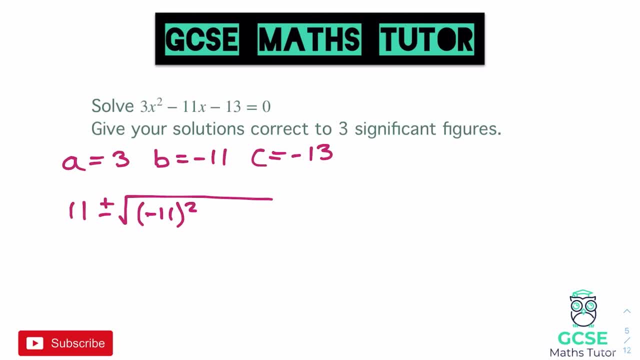 it will square the 11 and then put the negative sign within. you can test that on your calculator. if you just type in negative 11 squared, you'll get the answer negative 121. but we already know that negative 11 multiplied by negative 11 makes positive 121. So you need to be very careful. 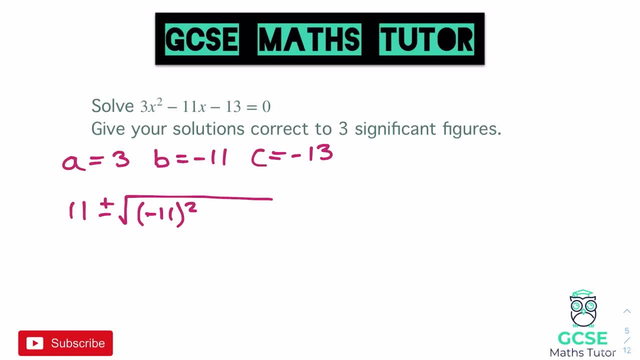 with that and do make sure that you put that into the calculator. I'm going to start typing this in as we go. So, plus the square root brackets, negative 11, close brackets squared, and then we're going to take away 4 times, 3 times negative 13 on the top. Just type that in: take away 4. 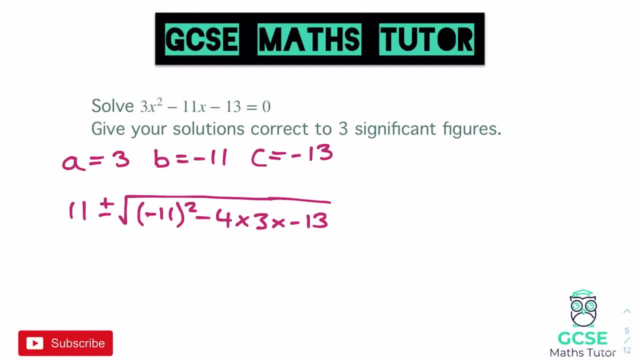 times 3 times the negative button with the 13. On the bottom: all over 2a, so all over 2 times 3,, which is 6. And let's type that in And with the plus sign, this time we get 4.607,219,496. 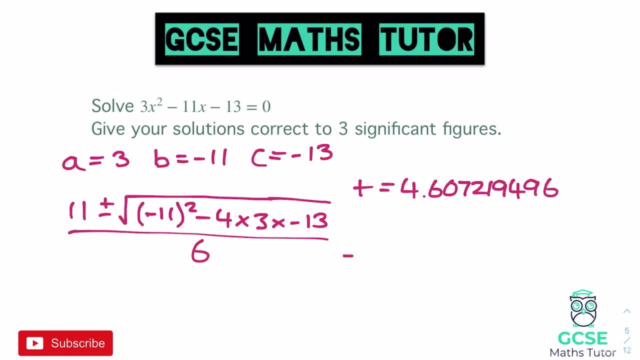 And again we'll round that to three significant figures in a sec. Let's go back in and get our negative version. So change that for a minus. There we go, Press equals again And we get negative 0.9405528295.. 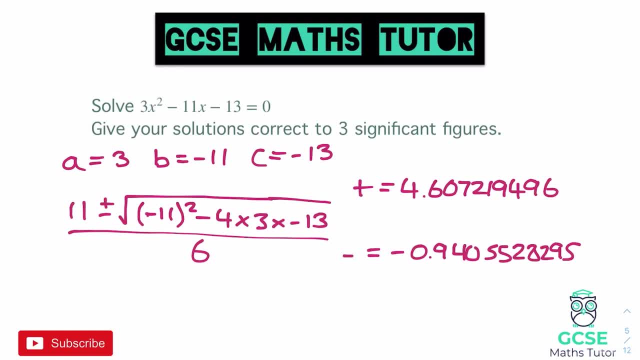 There we go. So again, rounding these to three significant figures, chop after the zero there and we get 4.61 for our first one, And then for the next one. here, that's 940.. So drop that to the zero and we get negative 0.941.. And there we go. There's our two solutions. 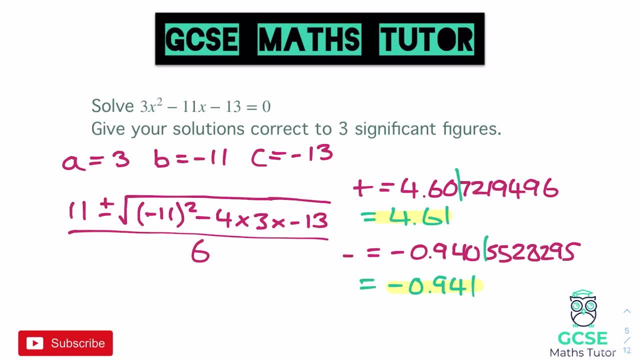 So, as you can see, the whole process is the same. You just need to be careful. When you have a negative b value, our first value here becomes positive, And also it's essential that this goes into a bracket. Thinking about it technically, you could just put positive 11 squared in that part. 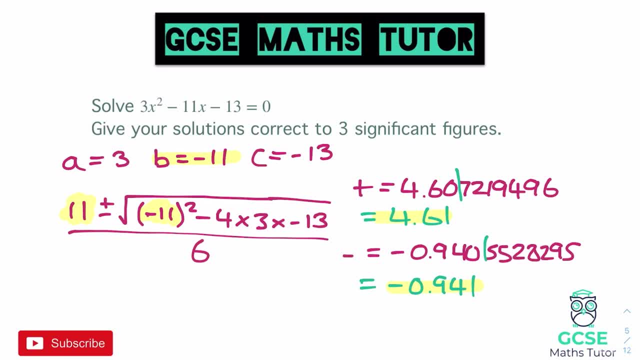 as it doesn't really matter whether we're squaring a positive or a negative version of the number. We still get the same answer. We could bypass this bracket by just putting 11 squared, But I think it's best just to show that you actually know which number you're actually substituting in and getting used to that process. 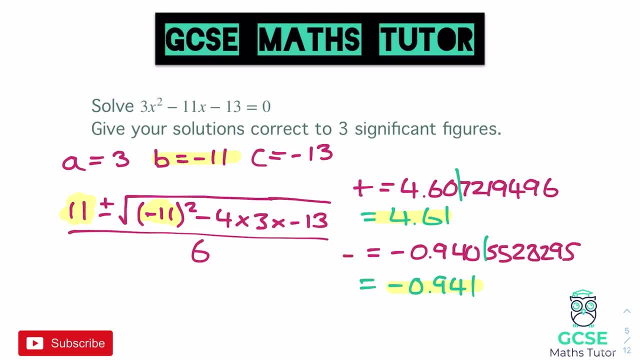 of putting negative numbers in brackets in your calculator. But there we go. There's our two answers. Same process, just obviously being careful with the negative b value. Let's have a look at a question for you to have a go at. Okay, So here's your question to have a go at. So pause the video. 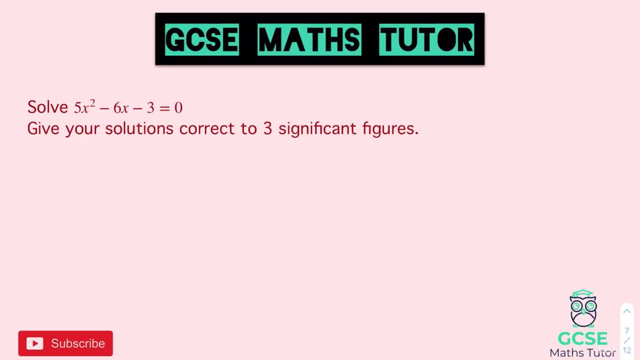 there. Have a go at this one, and we'll go over the answer in a sec. Okay, So, looking at this, then, our a value is 5.5.. So we're going to have a go at this one, And we're going to have a go at this one. 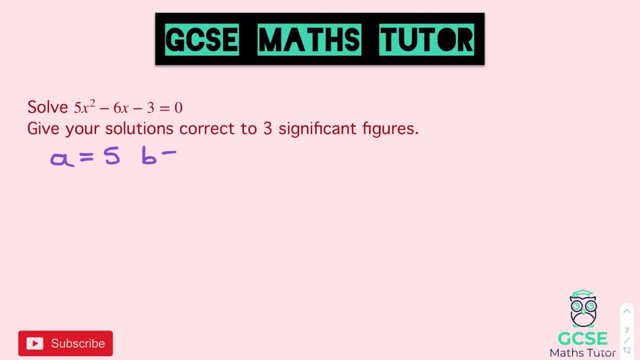 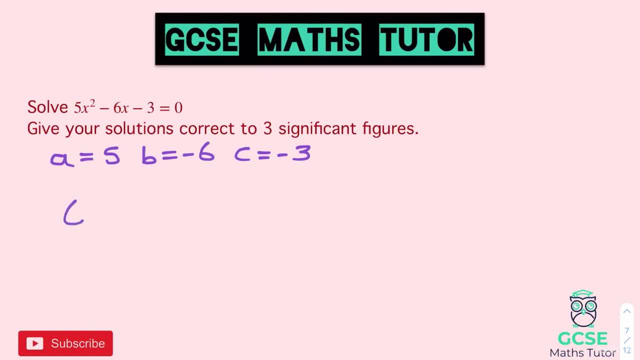 our formula again, the b turns into positive this time. So we have 6 plus and minus, And then we'll get our square root sorted. So we have negative 6 in brackets squared. Take away 4 times 5 times the negative 3. And that's all over 2a. It's all over 2, lots of 5, which is: 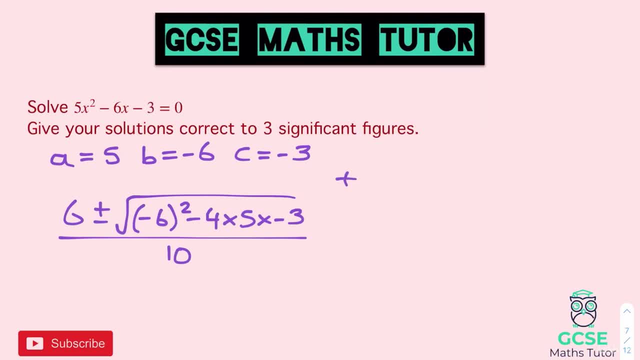 10.. Right, There we go. So we get our positive value, And in a sec we'll get our negative 1. So there we go, Let's put this in. So, for our positive value, let's put it in: So: 6 plus square. 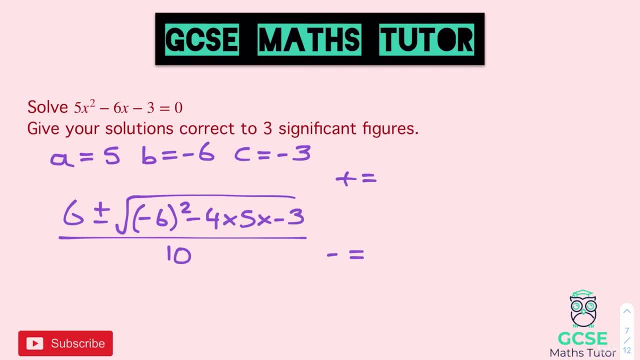 root of in brackets: negative 6 squared. Take away 4 times, 5 times negative 3.. And on the bottom we have 10.. So our value there comes out as 1.5.. Negative: 7.29,, 7.9,, 5.897.. And let's go back into the calculator. change the plus. 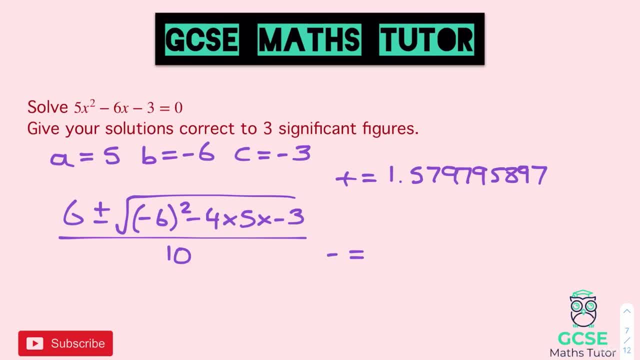 for a minus And we get an answer here of negative 0.379. And then 7.95. And then 8.A, 25. And then 8.9.. negative 0.379. And then .1.. That's the bottom. So we've got. the plus, So we've got. 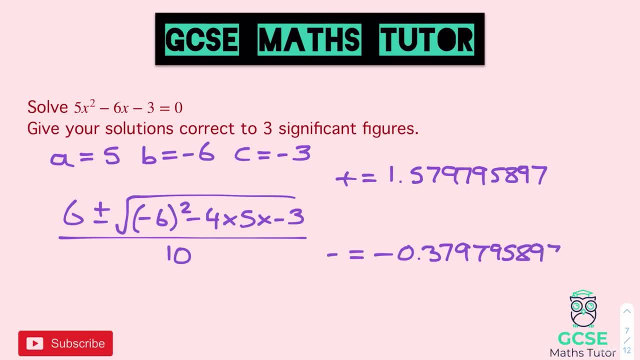 a plus, So we've got a negative. So there we go, And then we also have this plus, and then eight, nine, seven. one. there we go, and again we're going to round these to three significant figures again. so one, five, seven, and then we've got nine after that, so that's going to be one, five, eight. 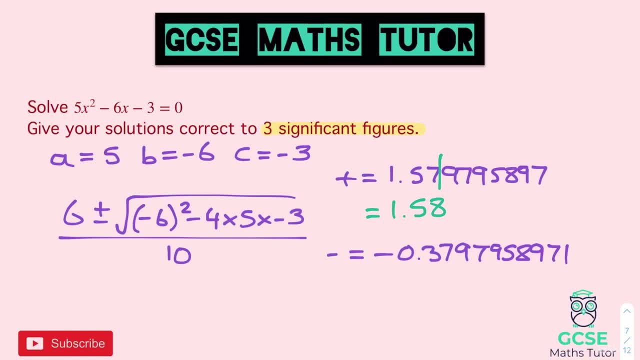 so one point five, eight, and for the one below three, seven, nine, and that seven's going to round the nine up. this is always an interesting one, because we get minus naught. point three, and that nine rounds the seven up, so it's going to be eight. and then, to make sure, we get our third, 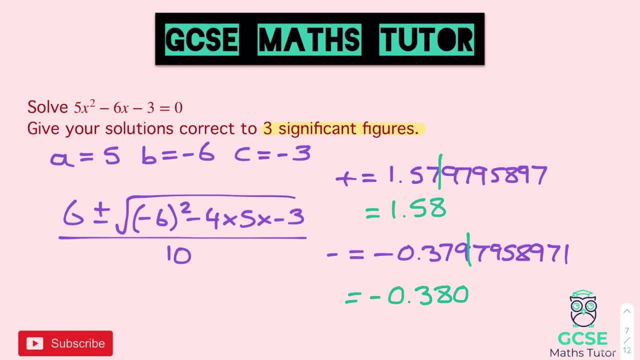 significant figure in. we'll emphasize the zero at the end there. so it's naught minus naught point three, eight, zero. right, there we go. so there are our two solutions: one point five, eight and negative naught point three, eight, zero, again not forgetting to emphasize that third significant figure, even if 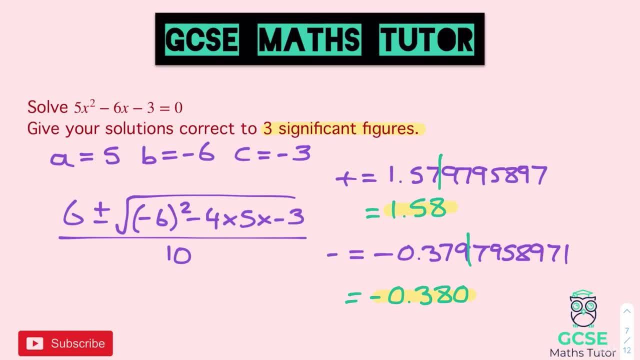 it is a zero. but there we go. there is our quadratic formula, obviously looking with a negative b value as well, and there's our two solutions. hopefully you're okay with those. now we're going to have a look at some quadratic formula, not using a calculator, and hopefully you'll see that's not. 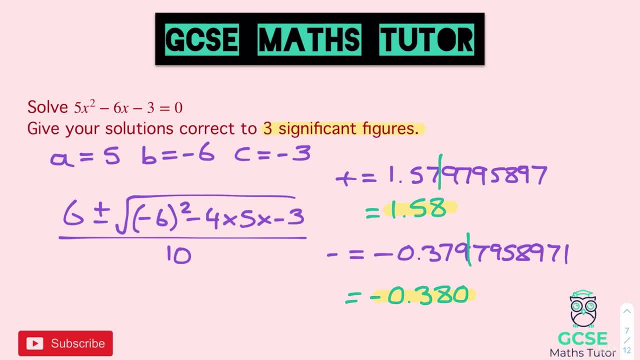 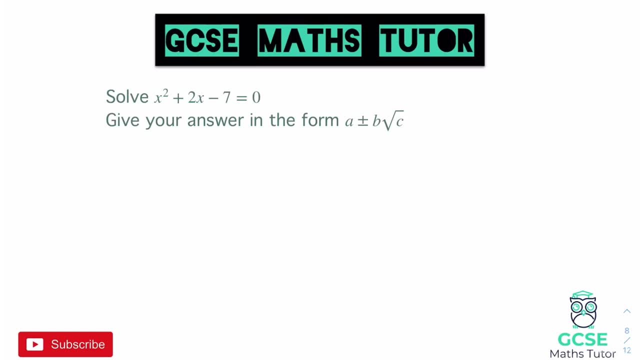 actually a quadratic formula. so we're going to have a look at some quadratic formula and we're going to have a look at that one now. okay, so for this question here it says: solve x squared plus two, x minus seven equals zero, and give your answer in the form a plus and minus b root c. 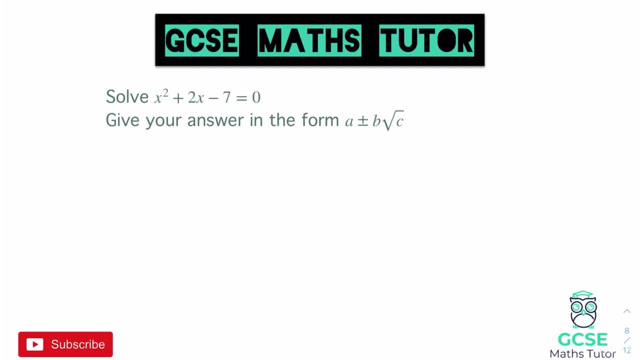 now, as you can see, it doesn't specifically say: obviously it's non-calculator, but this is a non-calculator style of question, so we're going to be doing this without a calculator. now, the little hint here is that it gives us the answer, it wants the answer and what we call. 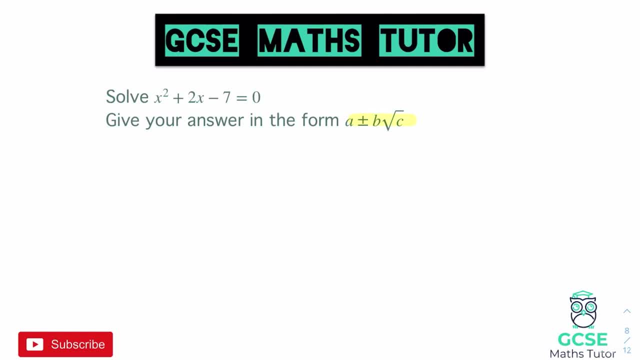 third form. so obviously what i'll do is i'll link some videos in the description, because you're going to need to be good at simplifying thirds for this one, so it's only the part one in the third series, but again, i'll link that in the description. but you're going to see at some point we're going. 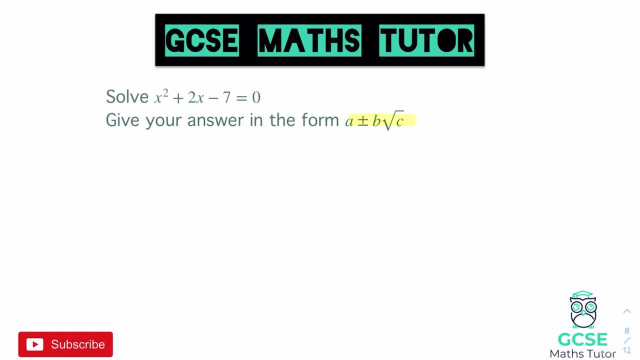 to have to simplify a third and the little hint there is we have b root c, okay, and that's a simplified third format. so we're going to have a look and see how we approach this, but for the majority, this we're just going to take exactly the same approach, so we get our a, b and c value. 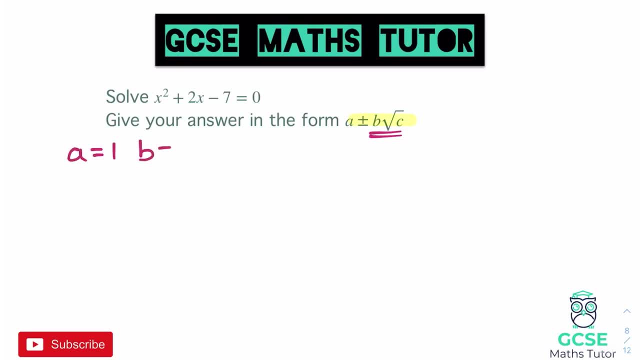 so a is one, b is the two and c is going to be negative seven. and again we're going to put that into the quadratic formula. so we have minus b, so minus two, and we have plus and minus the square root of b squared, so two squared minus four times a, which 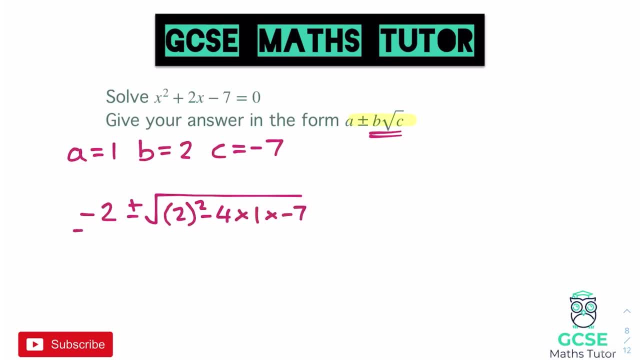 is one times c, which is negative seven. that's all over two a and two. lots of one is just two. so that's what that's going to look like now, what we need to do. obviously, we don't have a calculator, so we're going to take this bit under the square root and we're going to simplify all of that. 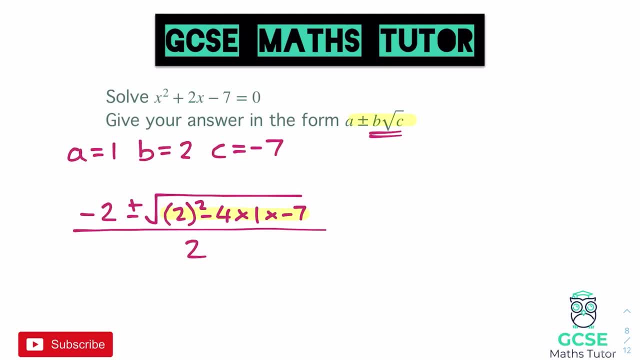 and let's just think about what that simplifies down to. so if i write this to the side, we'll get rid of it in a sec. we've got two squared minus four times one times negative seven. so to start, as two squared that's four, so we have four and we're going to take away four times one times. 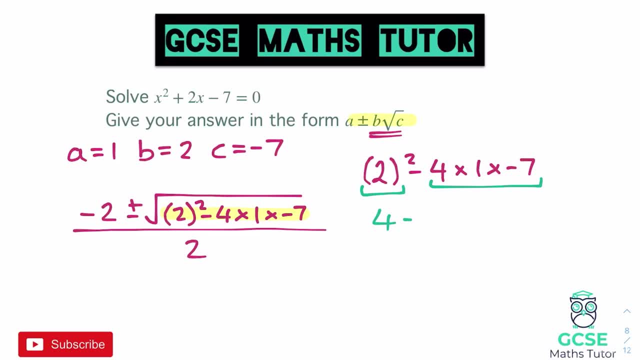 negative seven. well, four times one is four times that by negative seven is negative 28. so we have four. take away negative 28 and there we go. we've got that double negative there. so four take away negative 28 becomes four plus 28. so that's going to become 32. so underneath that square root we are going to have 32. so let's. 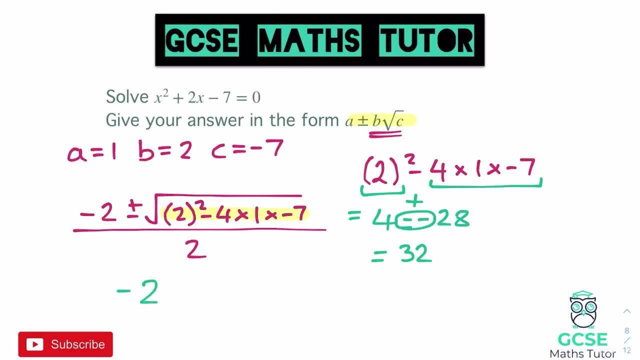 write this out with a 32 then. so we have minus two plus and minus the square root of 32, all over two. there we go. let's get rid of some of that working out to the right there so we can start having a look at getting this. 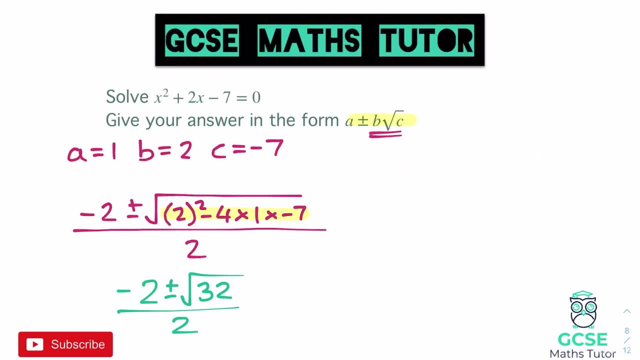 into our final form. now there we go and we have got an answer there. we've got minus two, plus and minus root 32 over two and we have actually got our two solutions there. we've got negative two, add root 32 all over two and we have minus, minus two. take away root 32 all over two. but again, it 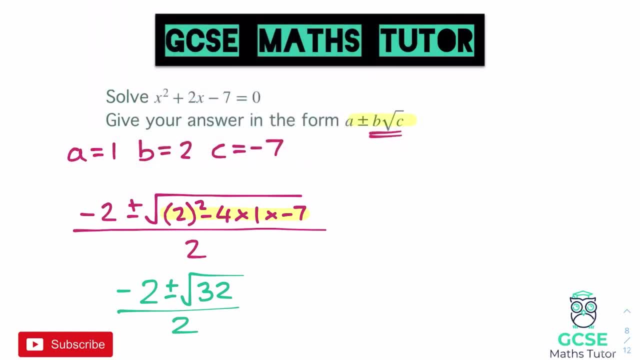 wants our answer in this form here, where we have a plus and minus b, root c, so no fraction involved. now, at the moment we can't divide everything by two. we've got the two on the top, the negative two. that divides by two, but at the moment we can't divide this root by two. okay, there's. 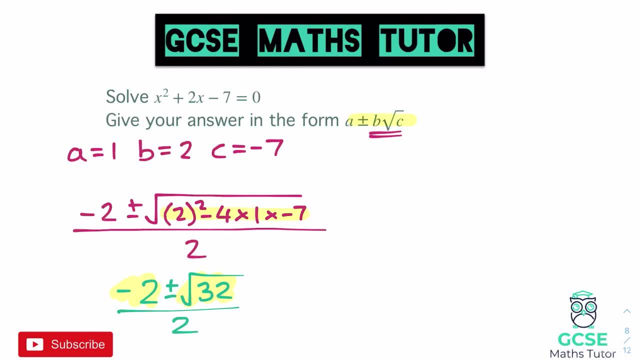 no number in front of the third. so if we can simplify this- hopefully- and it will, but hopefully- that number in front of the root 32 will divide by two and we'll just be able to simplify it all down. so let's have a look: root 32- and this is where your simplifying thirds comes in- root 32 can be. 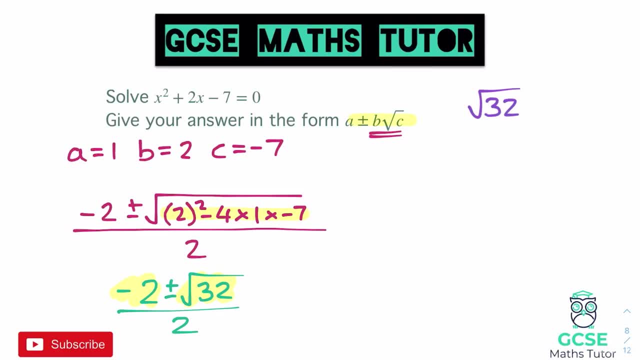 written in a different way. so again, thinking about thirds and checking out the description, if you're not okay with this bit. we're thinking about the two thirds that multiply to make 32, where one of them is a square number. now four is an option, but we want the biggest one and that's 16, so it's root. 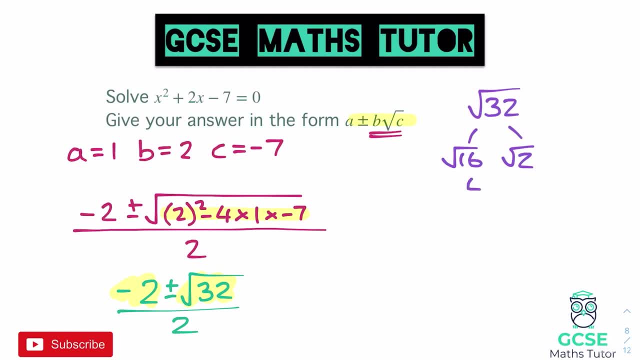 32 divided by root 2, root 16 is 4, so it becomes 4 root 2, so we can rewrite this root 32 as 4 root 2 and if we do that we have minus 2 plus and minus 4 root 2 all over 2, and now you can see the 2 here. 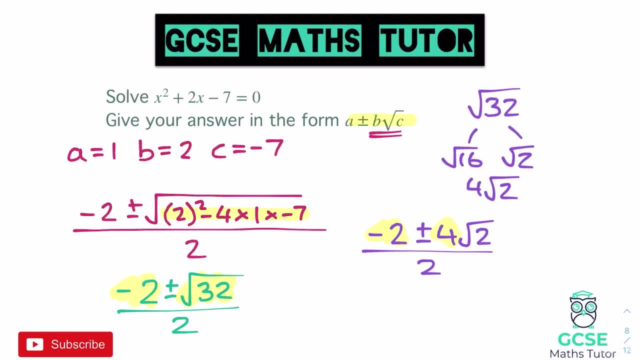 the negative 2 divides by 2 and also the 4 divides by 2. the root itself won't divide down. obviously, numbers divide numbers and the only thirds divide other thirds. but we can actually simplify this down now, so all we need to do is divide both of those by 2. 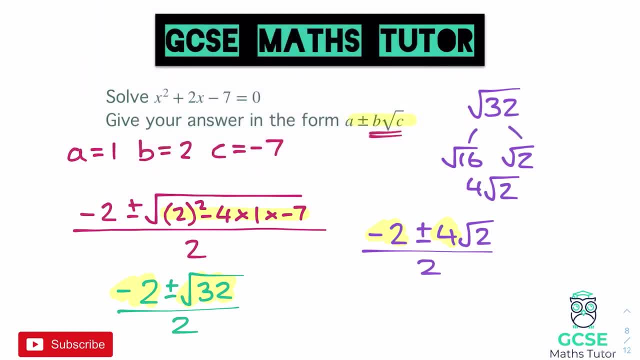 and we'll have our final answer there, and let's do that. so negative 2 divided by 2 is negative 1, and then we've got plus and minus. the 4 divided by 2 is 2 and then the root 2, so we have negative 1. 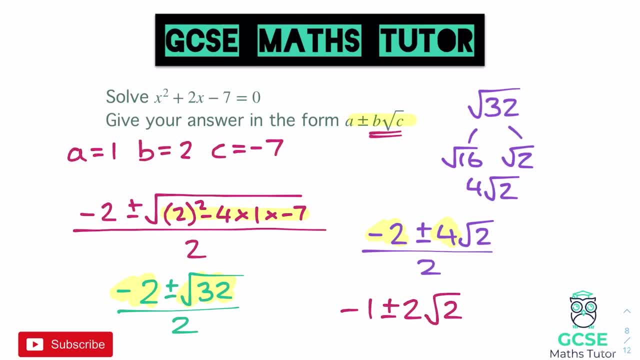 plus and minus 2 root 2. so, in terms of our format up there, a is negative 1, b is the 2 and c is also 2, and there we go. there is our final answer: negative 1 plus and minus 2 root 2, right? so that's how we do this, without a calculator, the whole process. 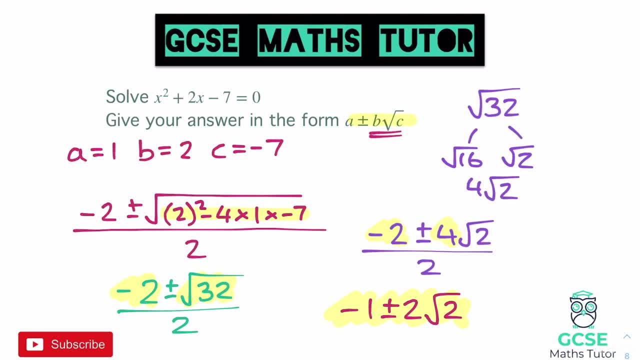 there is obviously looking at simplifying what's underneath the square root and for some of these questions- and i believe the next one that we're going to have a look at- you're going to have to also think about simplifying the third, so that we can divide it down by whatever numbers on the 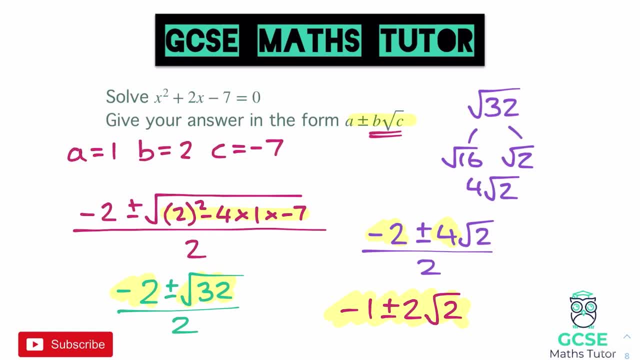 bottom, if we want it in this format. of course it might have asked for the format a plus and minus b, root c over d, or something like that, or just a plus and minus root b all over c, something like that, where it might have just wanted it in a fraction. if it didn't want it in a fraction, 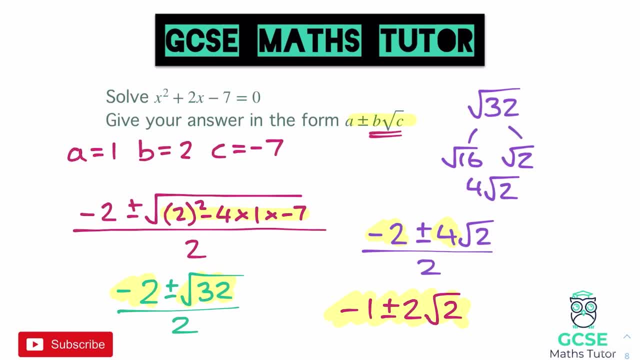 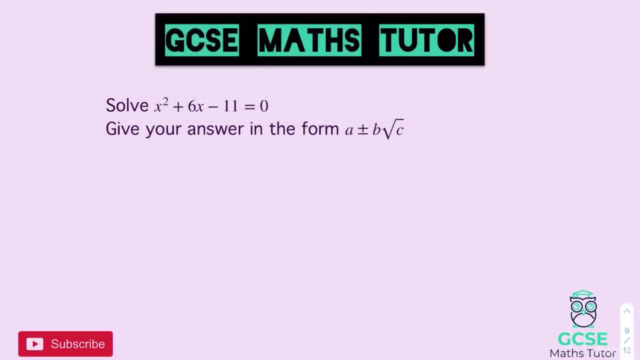 didn't divide down, but this is obviously just taking it that extra step and involving a little bit of simplifying thirds as well. so let's have a look at our final question for you to have a go at. okay, so here's your final question, obviously without a calculator similar format to what? 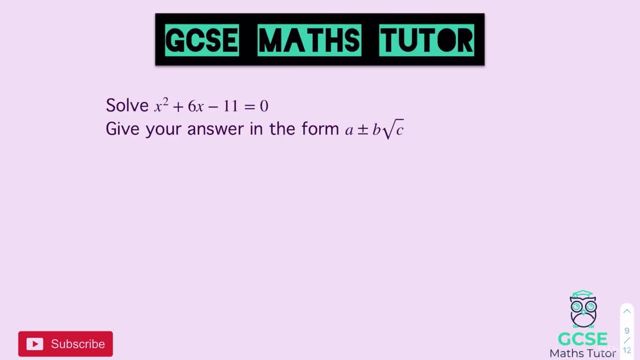 we were looking at last time, so have a go pause the video there and see how far you can get. okay, so for this one then. so our value of a is 1, our value of b is 6 and our value of c is negative 11, and if we plug all of that in, let's see what we get. 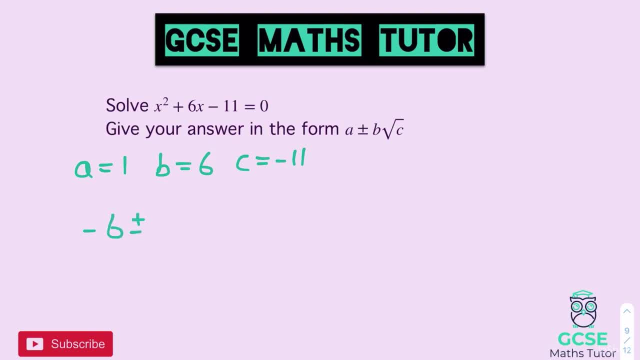 so we have minus 6 plus and minus the square root of, and then we have 6 squared minus 4 times 1 times negative 11, and that's all over 2a, which is 2. now if we just have a look at what's underneath the square root, 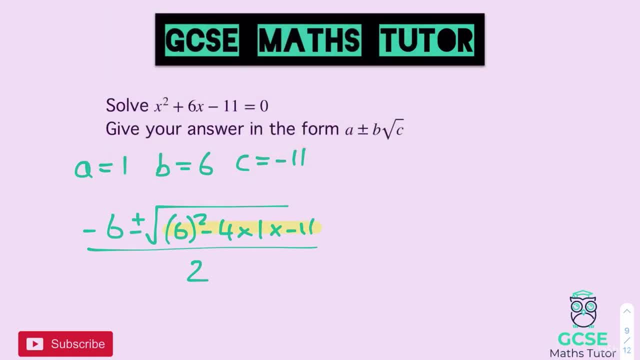 then- and we'll have a look at simplifying that down and underneath the square root- we're going to have 6 squared, which is 36. take away 4 times 1 times negative 11, which is negative, 4, 44. so 36, take away negative 44 is 36 plus 44, and that comes out as positive 80. there we go, so we. 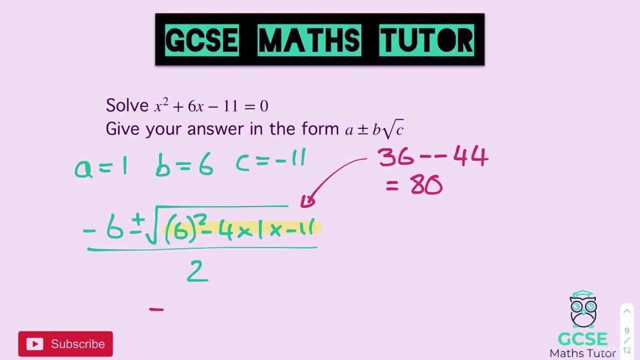 have positive 80. let's rewrite this then. so we have negative 6 plus and minus the square root of 80, all over 2, and again we need to simplify that root 80. so let's have a look at simplifying that. now, the square root of 80. let's have a look up here. 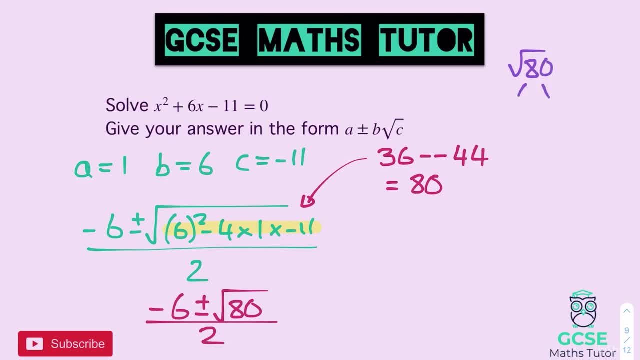 we can rewrite the square root of 80 as 4. we can see it rotates all the way back to. t equals the square root of 80. that's what we've actually done in oh. t also does look in here at, so let's bring this up and finish it off. so we have negative 6 plus and minus 4. 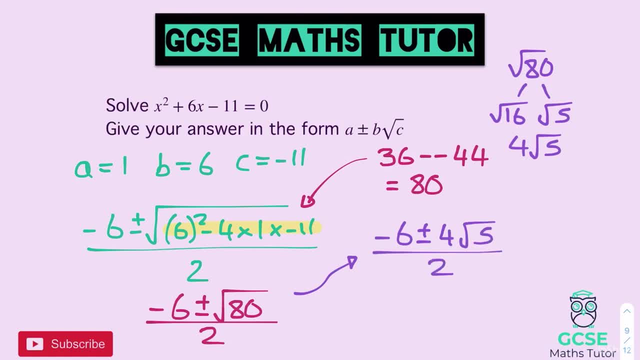 root 5, and that is all over 2. and again, we'll take the same approach. we'll divide this 6 by 2 and the 4 by 2, and that's going to leave us with negative 3 plus and minus 2 root 5. and there is our final answer with our final question. 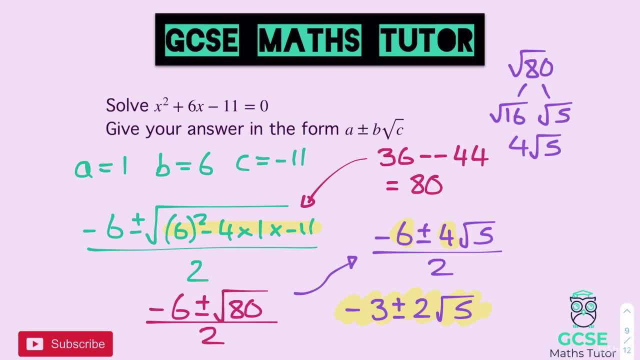 negative, 3 plus and minus 2 root 5, and that obviously just gives you a little bit of a showing of how you can actually use the quadratic formula without a calculator, but obviously we would leave our answer in this surd form. there is another unique scenario, in which case the number under the square 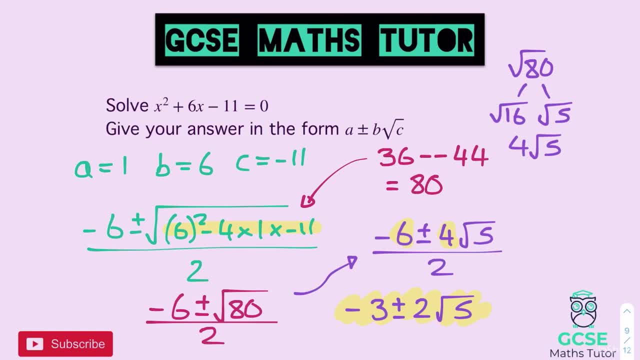 root could actually be a square number, in which case you could actually get some whole numbers out of this as well, but obviously that would indicate to you that you could have actually factorized and there would have actually been some whole number solutions within the brackets. so it tends to be that we'd 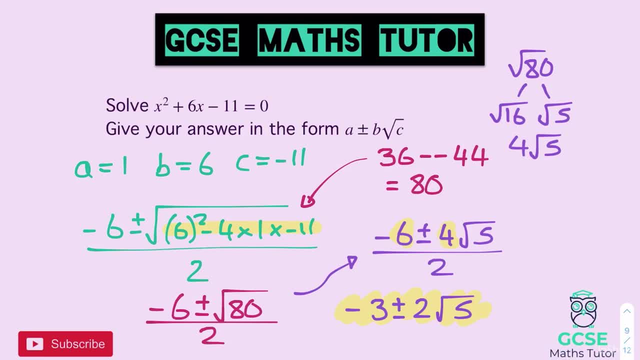 only use this process really if it doesn't factorize and obviously write our answer in surd form. but there's a little bit of a showing of how you can actually use the quadratic formula. there we go. there's some work on the quadratic formula, don't forget to. 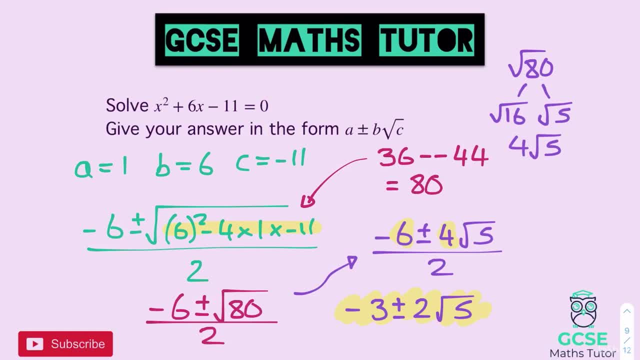 check out the rest of the series on algebra here and obviously looking at forming and solving quadratics, solving quadratics by factorizing and all those sort of other elements of quadratics that are within that series. hopefully found that useful and helpful. if you did, please like, please comment please. 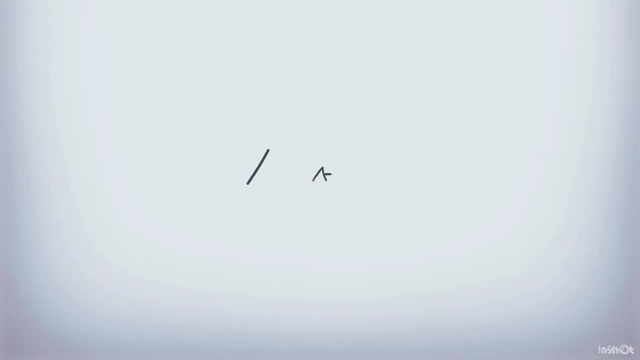 subscribe and I'll see you for the next one, you.